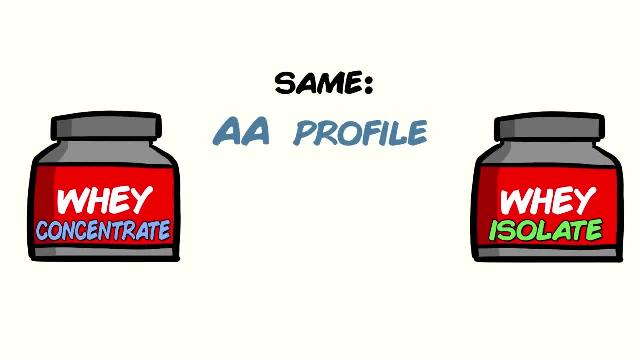 isolate, Both share the same amino acid profile and both have extremely high levels of absorption and digestibility. Both have the same immunoglobulins and lactoferrins that are good for general health. In terms of fitness, both whey protein variants and protein in general can aid in exercise recovery. 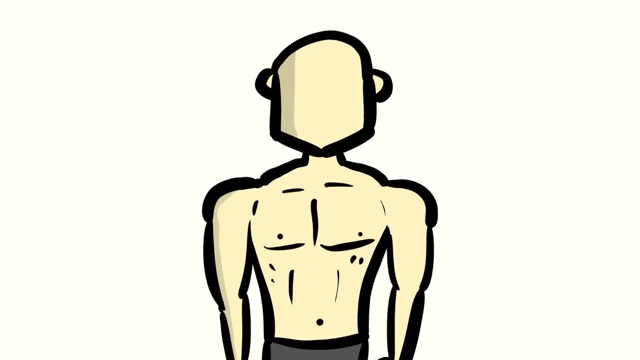 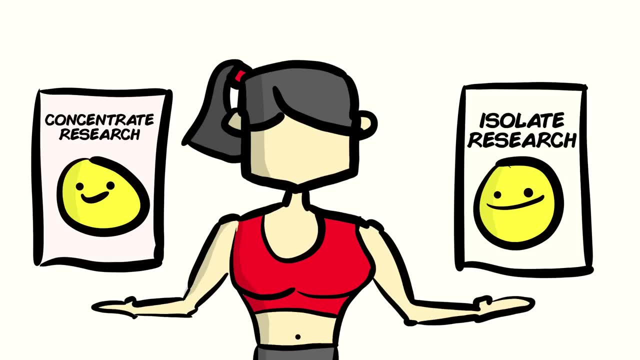 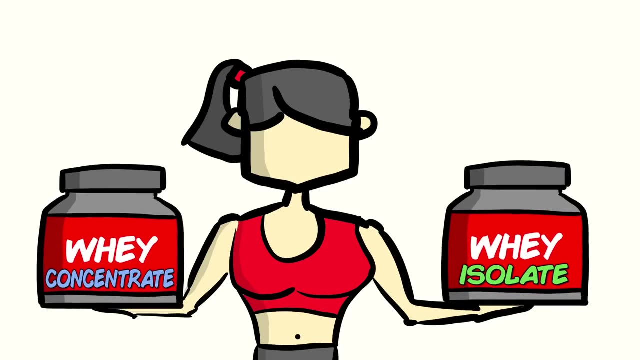 with no data showing one being better than the other In terms of body composition. well, unfortunately we don't have much research comparing the two directly. What we do have is plenty of data looking at each separately and comparing them to isocaloric controls, And when it comes to this again, both seem to get the job done. 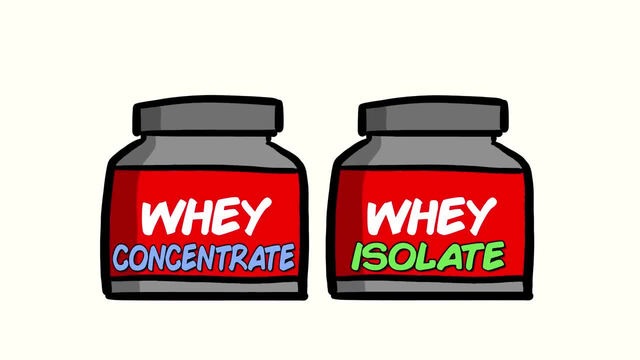 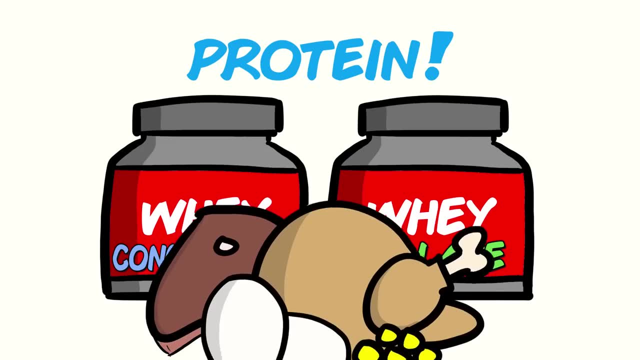 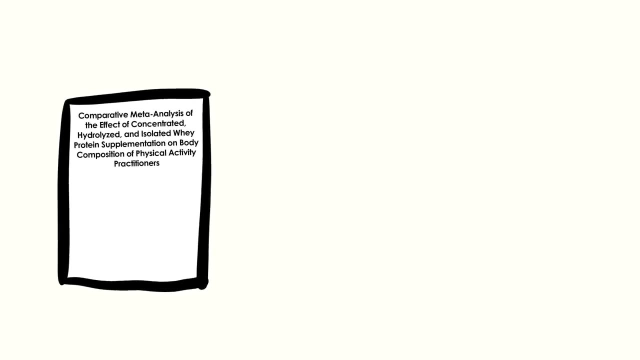 just as good as the other. In essence, they are still what they are. Protein Total protein intake, be it from whey concentrate, isolate or just whole foods, is what matters most Now. a systematic review just released this year- 2019, did find that, after investigating 8 different whey protein, 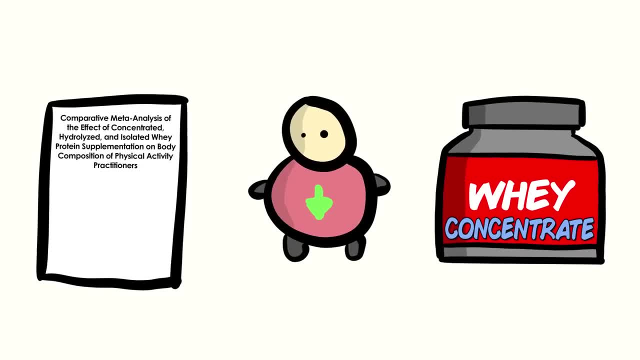 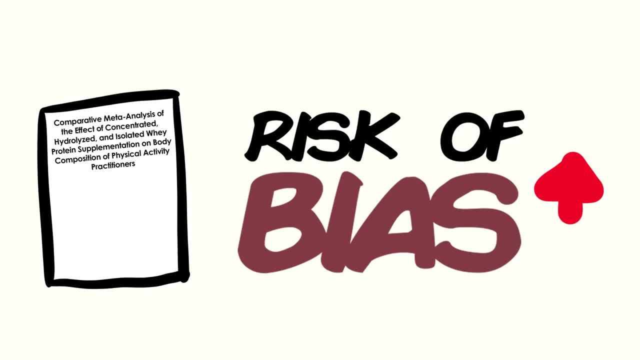 studies for fat loss whey concentrate actually had an upper hand, But the researchers did make it clear that these studies did have a very high risk of bias due to low methodological quality And, honestly, they were saying that these studies might have unintentionally implemented. 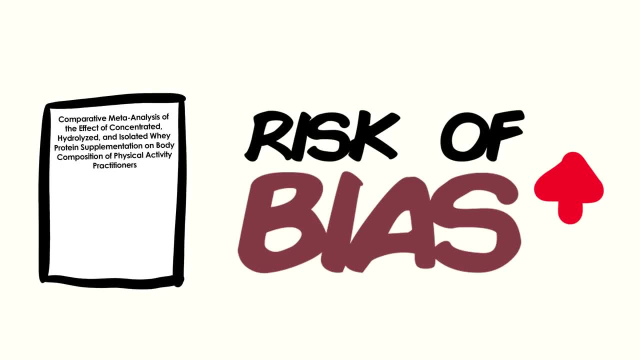 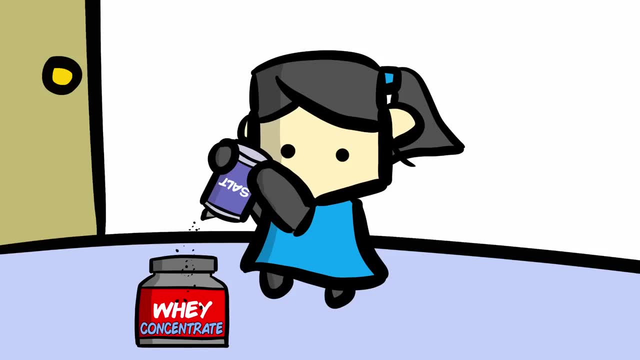 experimental practices that would have jeopardized objective results. So we should tick the findings of greater fat loss from whey concentrate with a very big grain of salt. Now to answer the question: which whey concentrate or isolate should you take? 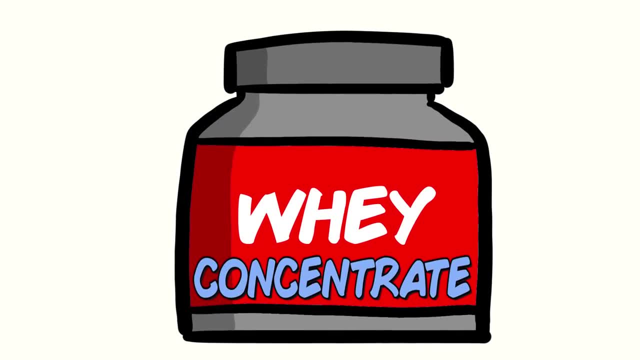 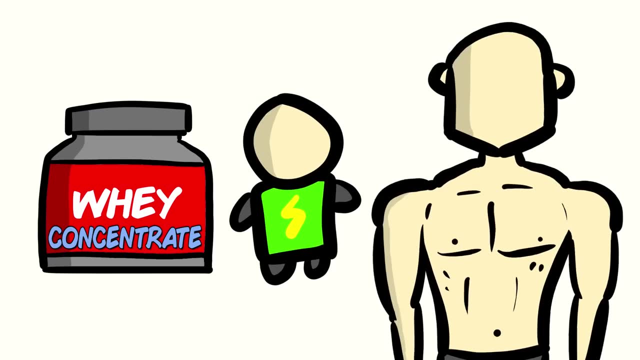 When we take everything into consideration, whey concentrate makes the most sense for most people. It provides virtually the same fitness benefits as isolate, both in recovery and muscle growth. And, of course, whey concentrate is the most common type of protein in the 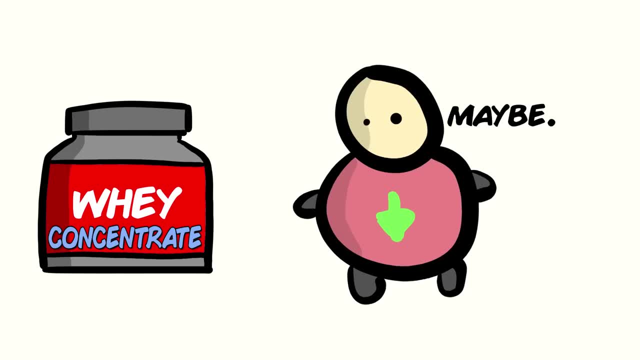 world, And in the case of isolate whey concentrate is the one that can be used for most purposes. However, it is usually less expensive. Now there are some still cases where whey isolate makes more sense. Remember, whey isolate. 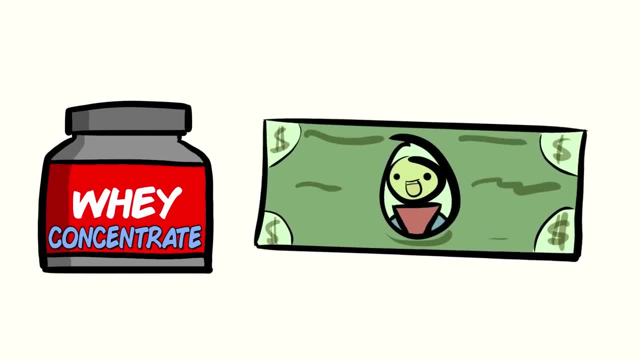 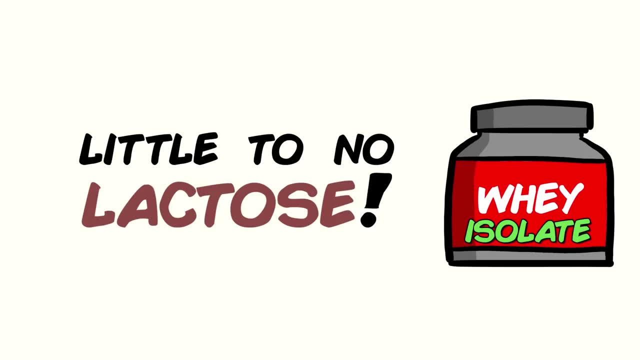 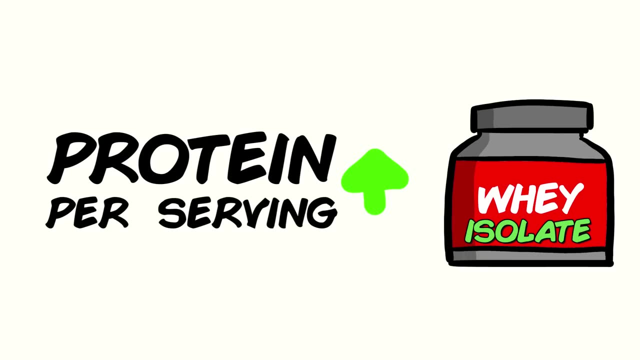 has little to no lactose, which is perfect for those dealing with any degree of lactose intolerance. Whey isolate also has more protein per serving For those, especially athletes, that need to meticulously account for every gram of protein in their supplements. then whey isolate. 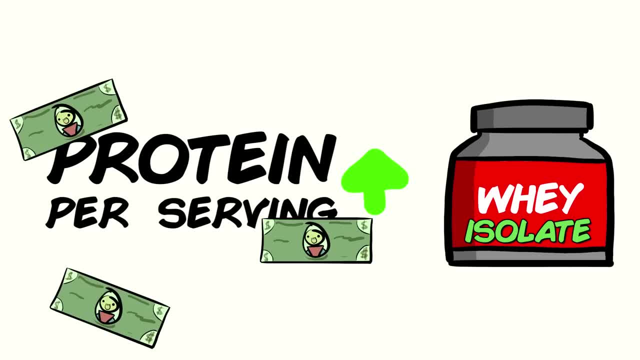 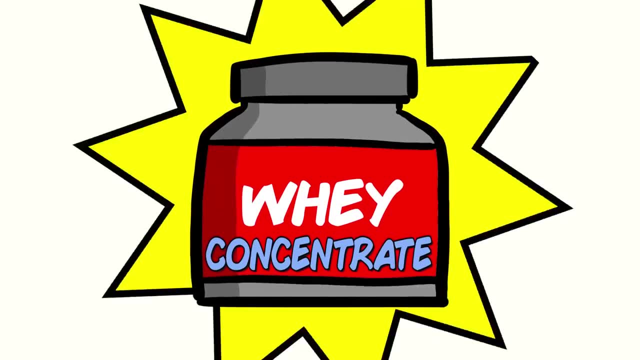 is the better choice. So, in conclusion, whey concentrate is the best option for those who are looking for that. you will have to spend a bit of a premium for the small differences. For everyone else, again, concentrate should work just fine.